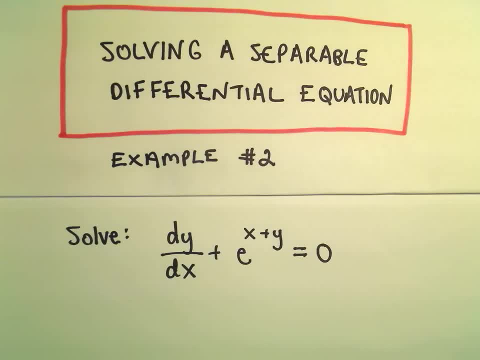 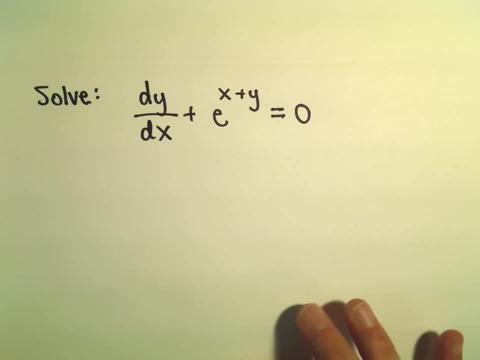 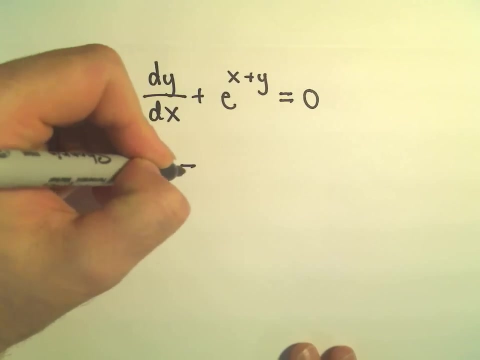 Alright, in this video I'm going to solve another differential equation. So here we're going to solve dy. dx plus e to the x plus y equals 0.. And again, with a differential, a separable differential equation, we kind of want to put the x's on one side and the y's on the other. You know, obviously it doesn't matter which side which is on. So I'm going to start off by writing this: dy over dx. I'm going to subtract the e to the x plus y to the right side. So I'll 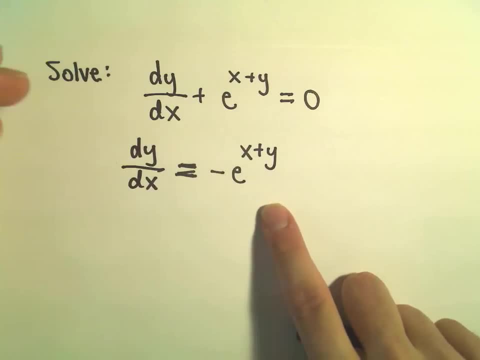 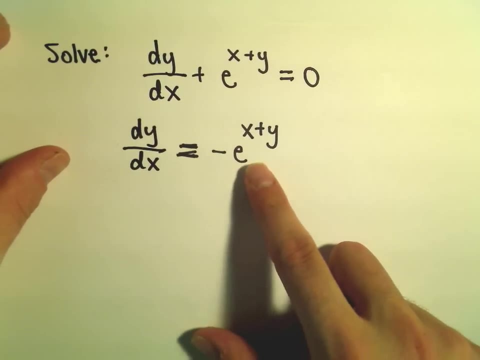 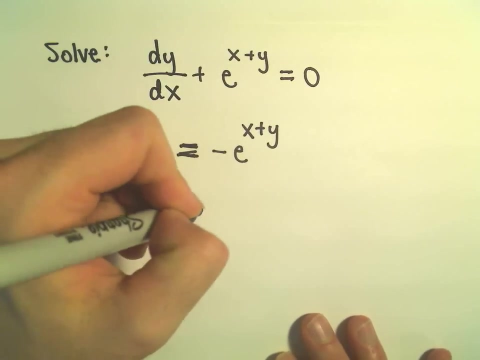 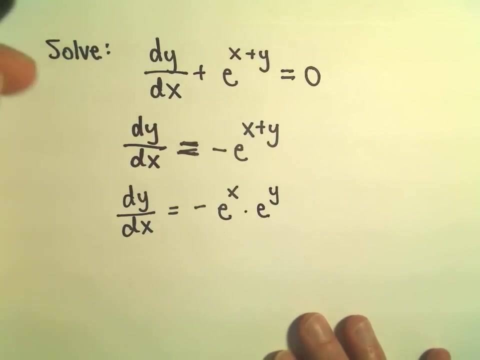 get negative e to the x plus y. So again, somehow we have to get, you know, all the y's on one side. So we're going to have to somehow, you know, break this thing up. And the way that we're going to sort of break it up so that we can move things around is, well, I could write e to the x plus y as e to the x times e to the y, right, If we have like bases, we would add the exponents and we would get e to the 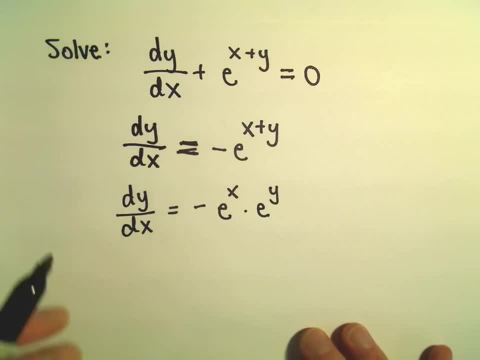 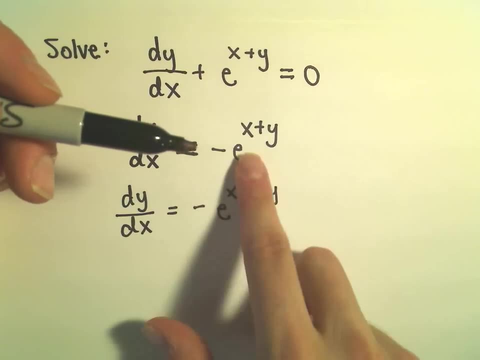 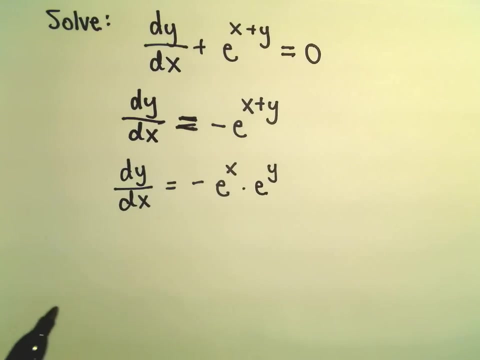 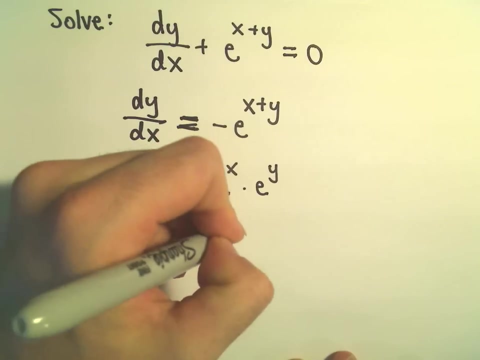 x plus y right back. So sometimes people, it seems like, get a little, you know, feel a little uncomfortable, don't quite recognize this. It's certainly common to have like bases and write them together, But again we can always, you know, sort of go backwards and break them up. So that's all we're doing here. Okay, so I'm going to multiply both sides here by my dx, So that's going to give me negative e to the x times e to the y times dx. And now I want to get 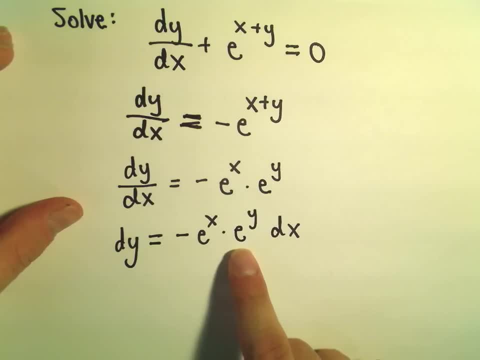 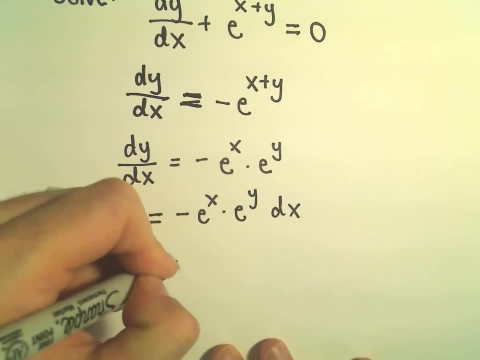 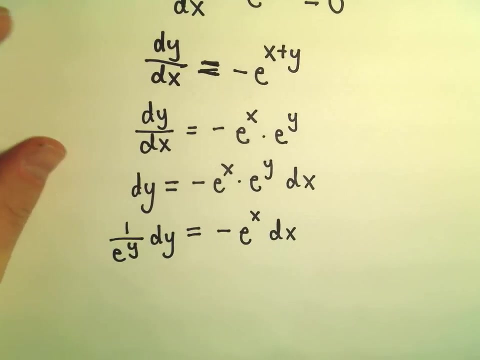 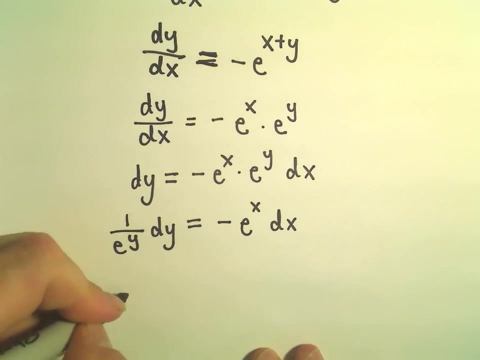 again sort of the y's over to the left side. So I can simply divide both sides by e to the y And I'm going to write that as 1 over e to the y dy. We've got negative e to the x dx And I'm going to do one more thing. So because eventually I mean our goal here is to integrate this, So the 1 over e to the y, I'm going to write that as e to the negative y dy And then we've got negative. 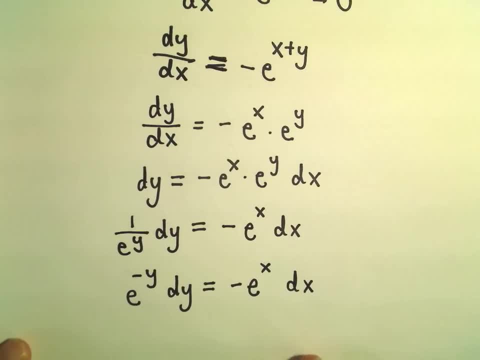 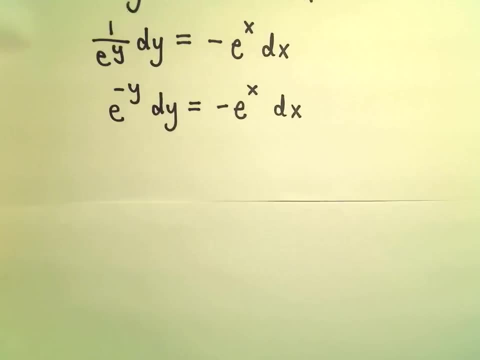 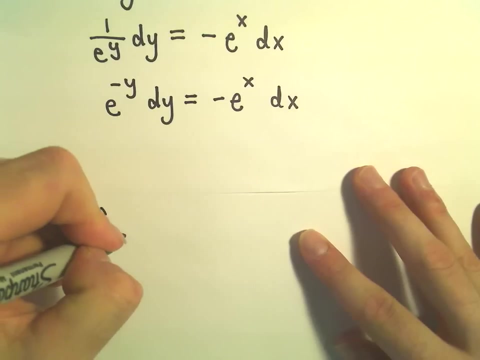 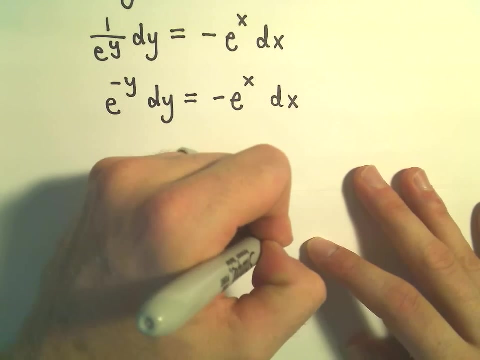 e to the x dx. And now this is kind of a good place. Things are separated out. We've got our y's on one side, We've got our x's on the other, So now we're just simply going to have to integrate both sides. So I'm going to integrate the left side, e to the negative y dy. I'm going to integrate the right side, negative e to the x dx. So to integrate the first. 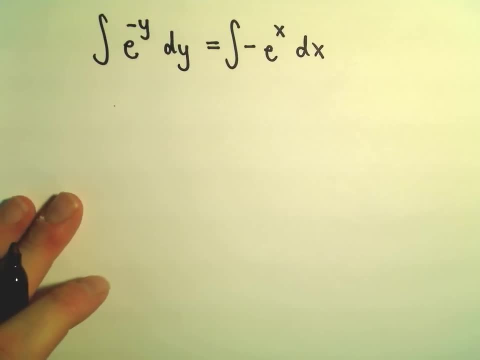 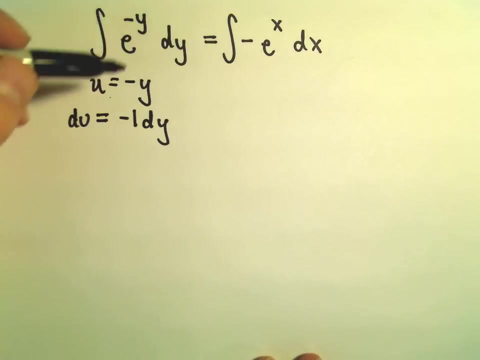 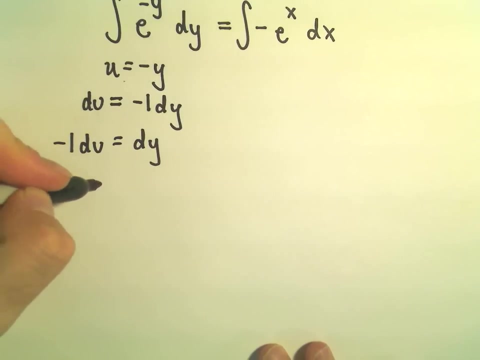 side. here, you know, these should be hopefully relatively straightforward integrations. On the left side we can do a u substitution. Let u equal negative y. du is going to be negative 1 dy And again I think you know we're replacing positive dy. So I'm just going to multiply both sides by negative 1.. So if we rewrite this we would simply get. we would have e to the u again because we're replacing negative y here. 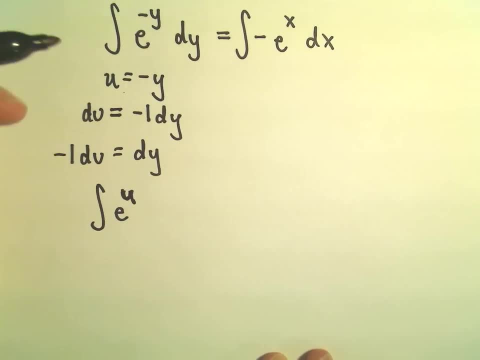 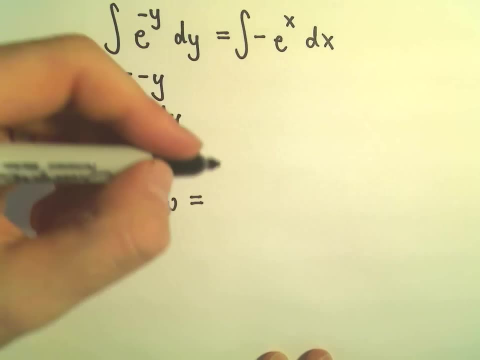 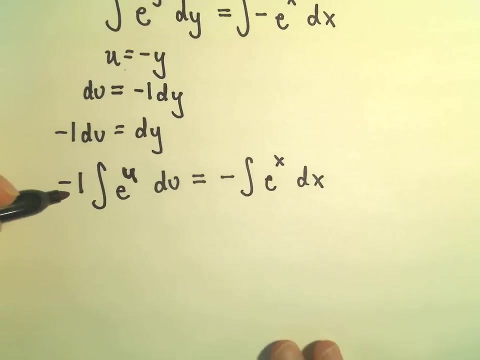 So we would have e to the u. dy is being replaced with negative 1, du. So I'm going to pull the negative out front. I'm going to do the same thing on the right. I'm just going to pull the negative out front, And now we can integrate both sides. So on the left the negative 1 comes along. The antiderivative of e to the u is just e to the u. Again, on one side or the other, we just have to stick our plus c. So I always just stick it on the right side. 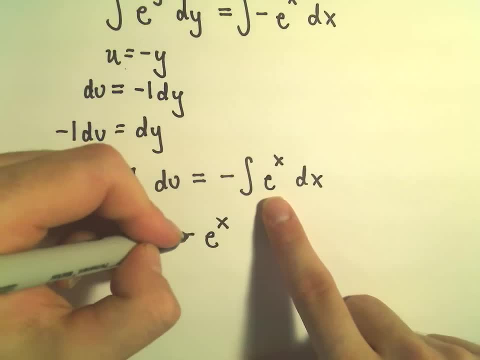 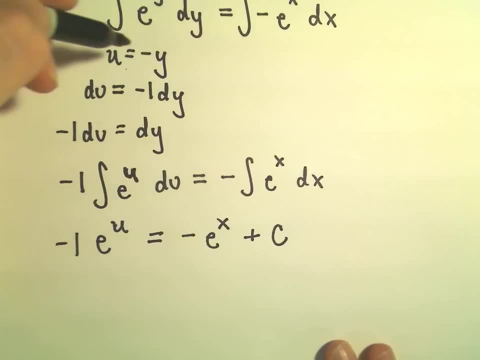 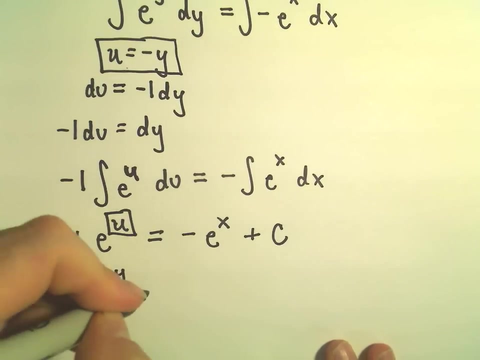 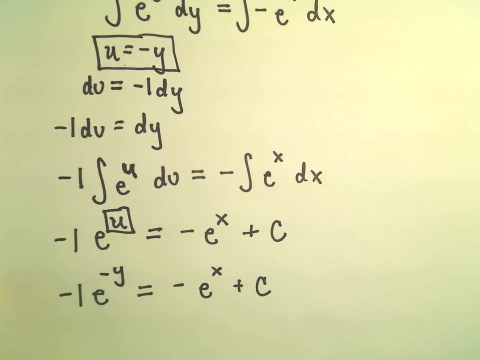 We'll integrate, we'll get e to the negative. well, excuse me, we'll get negative e to the x. I'm going to stick my plus c on that side. I'm going to replace again the fact that u here is simply equal to negative y. So I'm going to plug that in. So we'll get negative e to the negative. y equals negative e to the x plus c, And if we want to, we can multiply both sides here by negative 1.. So that'll give me e to the negative y.